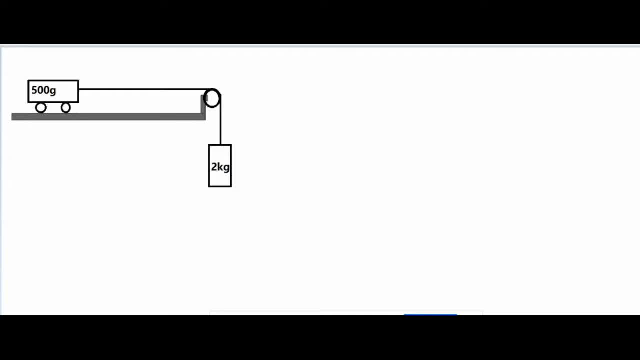 cart. So the first we want to do is we want to go ahead and draw our forces on each of the objects and then define a system before we set up some equations and then get calculating with some numbers. All right, so the first thing we're going to do is we're going to take a look at the cart. 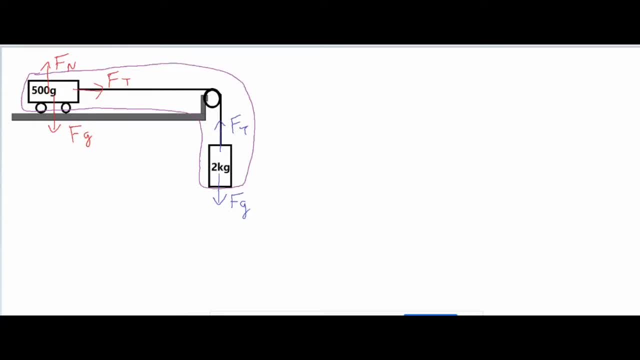 and for the cart, we just are going to assume that the friction force is small enough to where we can just go ahead and ignore it. If you want to see a case where the friction is significant, go ahead and click on the cart above. But for this scenario we're not too concerned about the force. 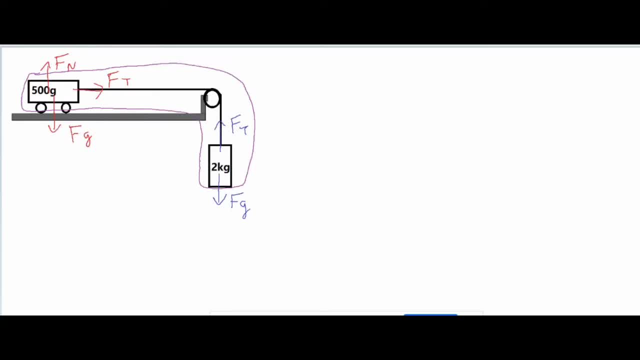 of gravity and normal force. These two are going to be equal and opposite. They're going to cancel each other out. and it's not along the axis of the direction of the cart. So we're going to take a that the cart is moving. So we have the ft, which is the net force, which means that it equals m times. 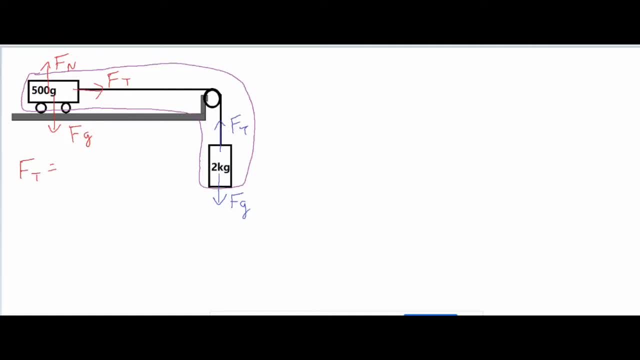 a. So before I write in 500 grams for the m, I want to make sure I convert it into kilograms. so I'm going to divide it by a thousand, which would make it 0.5 kilograms times acceleration, And then that's the only formula I'm going to need for my cart And then for my hanging mast. it has a. 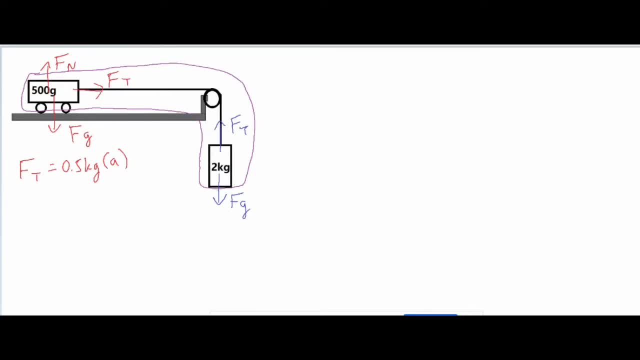 fg and then it has an ft. Now, before we get going with that, one thing we have to keep in mind is, when we have pulleys, it can kind of affect the positive and negative values, And what I mean by that is we have a system over here where a cart is being pulled and then the pulley redirects the force. 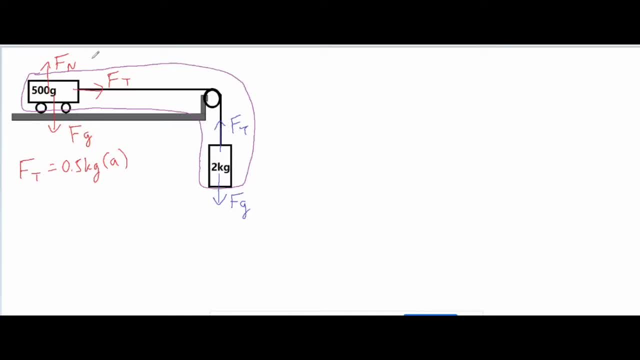 from this hanging mast and then goes downwards. So everything in the direction of the acceleration for the cart and the hanging mast would be considered positive. So typically you would say to the right is positive and to the left is negative which does hold up for the cart Over. 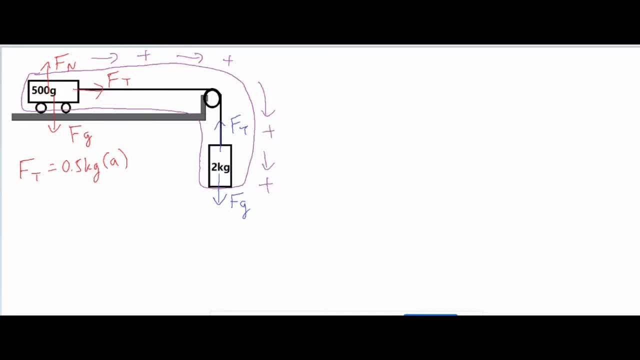 here a lot of times we would say downward is negative and then upward is positive. So that's going to be a little bit different. So we're saying everything along the direction of the acceleration for both the objects involved is going to be positive. So when I write my equation, 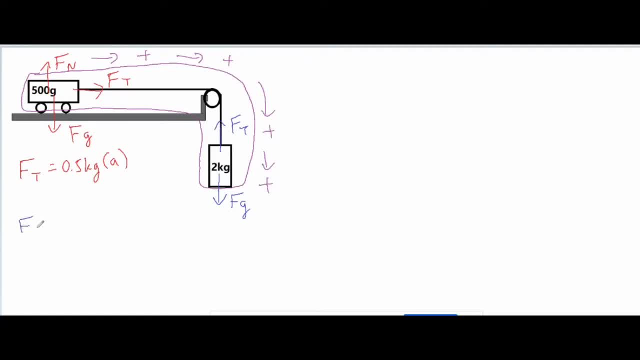 I'm going to say fg, and then I'm going to say fg, and then I'm going to say fg, and then I'm going to say fg minus ft, and I'm going to make my ft, my negative, and then I'm going to set that equal to. 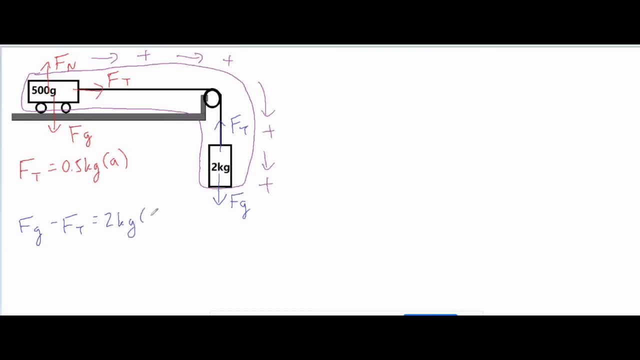 m, times a two kilograms, times that a right there, And then for our entire system. so our entire system is the part that I circled in purple. We only have one force, that's an external force that contributes to the acceleration. So we're going to say fg minus ft, and then I'm going to set that. 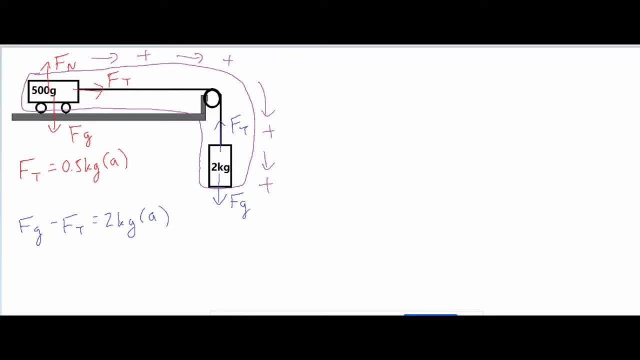 equal to m times a two kilograms times that a right there, And then for our entire system. so we're going to say fg minus ft and then I'm going to set that equal to m times a two kilograms times that acceleration of the system. So things that are internal forces aren't going to affect the 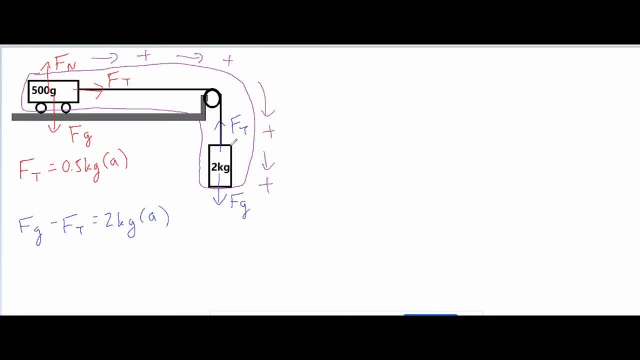 acceleration. So these are inside of my purple system. So my ft's don't matter, And my fn and my fg- they're going to cancel each other out anyways. So this fg is the only contributing factor to the acceleration of the system. So I'm going to go ahead and write fg. 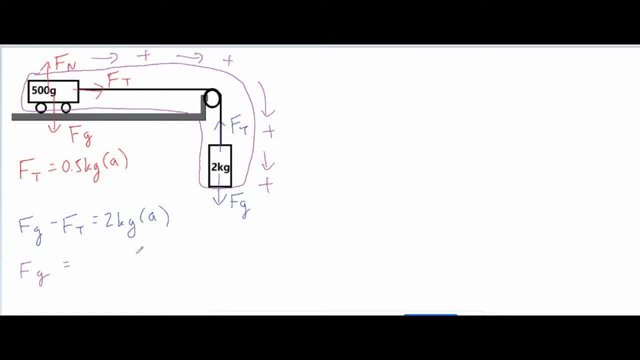 equals m times a for the whole system. So the whole system is going to be 2.5 kilograms. All right, so I have a set of three different formulas And the first thing I want to do is solve for acceleration, And if I take a look at what I have, I don't have enough t yet. 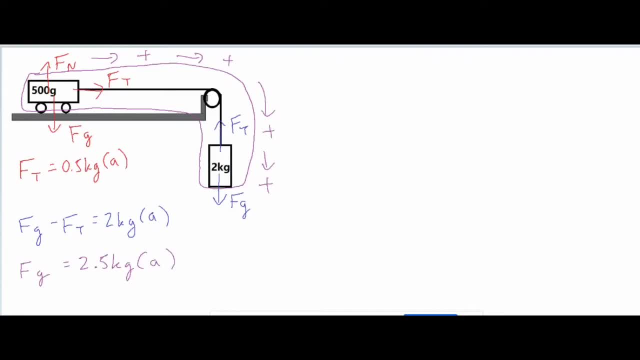 I don't have the a for my fg. I do have the fg, which is just two times 9.8 mg And that gives us 19.6.. I don't have ft, because that's the same ft as that one, And I don't have my a, So 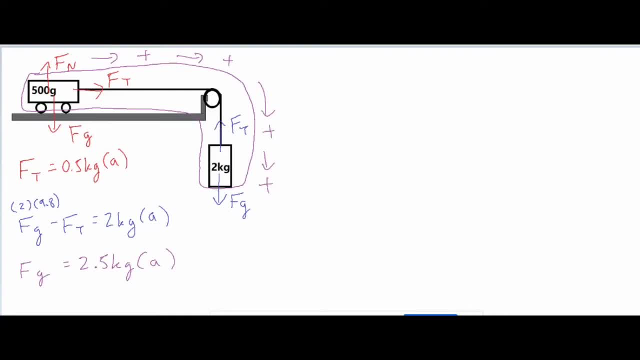 I'm going to go to my last one, my purple formula. And then this fg is the same as this one over here, which is the force of gravity on the two kilogram mass. This one, I do know everything except the a, which means I can go ahead and solve for my a with a little bit of algebra. 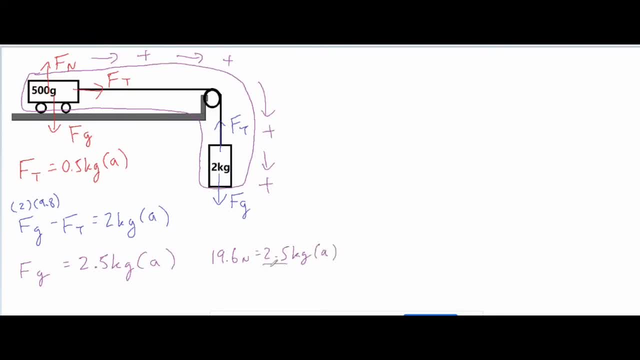 All right. so I went ahead and solved for my acceleration. I got 7.84 meters per second squared, which is pretty large for this kind of setup, But we do have a two kilogram mass hanging off the edge, So that acceleration is going to be 7.84 meters per second squared. 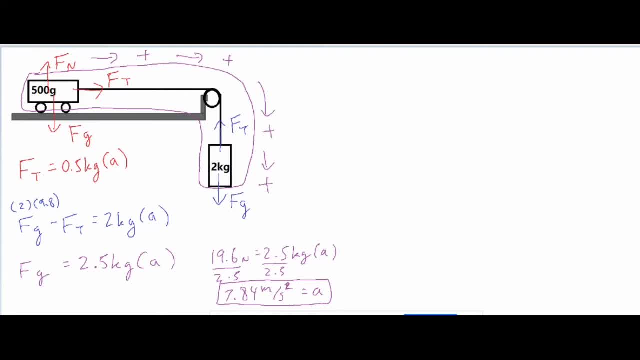 It's going to be pretty large. So we found our acceleration, And the second thing we're going to solve for is our tension. And for our tension we have two formulas which we can utilize. We have one up here and we have one over here. I'm going to go ahead and use this. 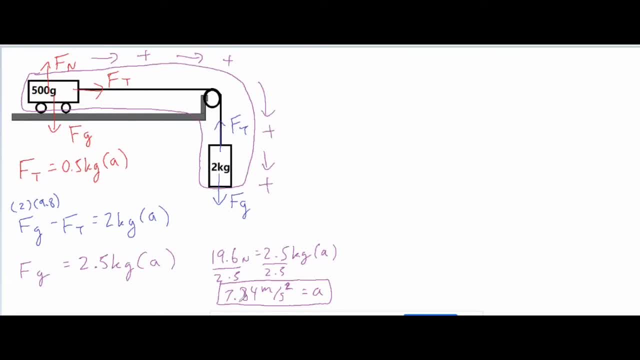 one over here, because this one looks a little bit more simple. So I know my acceleration is 7.84.. So if I go ahead and plug in the 7.84 over here, then my force of tension is 0.5 times 7.84 meters per second squared, which is the acceleration I just solved for. 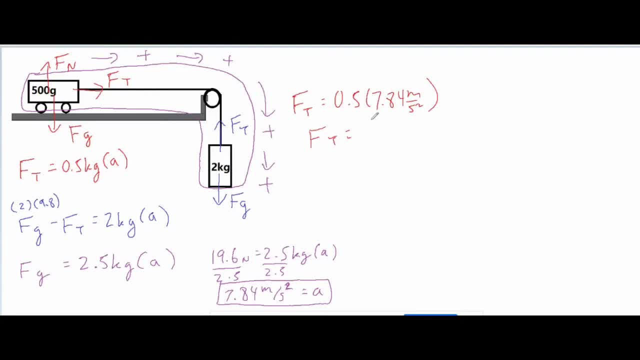 And then my force of tension comes out to be 3.92 newtons. So I finished the first portion of the video, which is solving for the acceleration and the tension, And for the second part of the video we aren't going to need this. 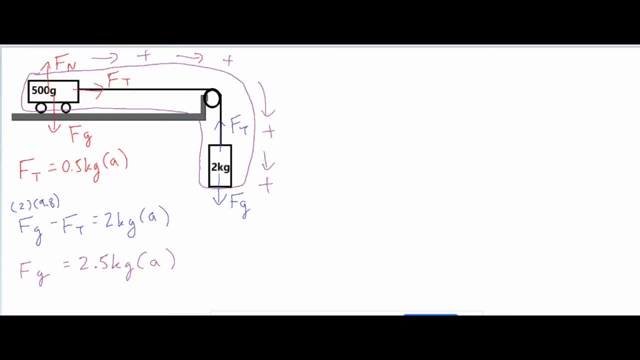 The second problem we're going to do is we're going to solve for an unknown mass that's sitting on top of our cart. So say, for example, we have a mass that's placed on top of the cart and we're trying to solve for that unknown mass based on some values that we're going to be. 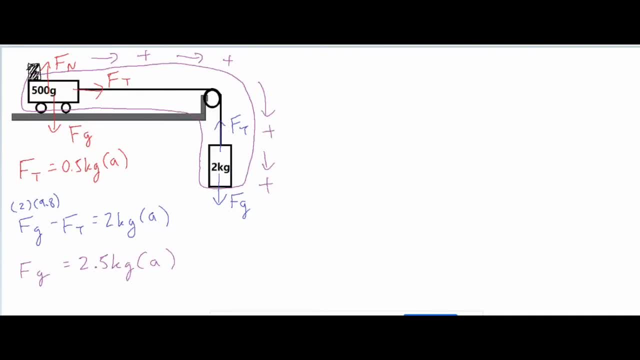 finding in the lab and by doing some calculations. So what you would typically do is you would use a motion detector And with that motion detector you would take a look at your velocity versus time graph And you would get something that looks like this: because you have a uniform. 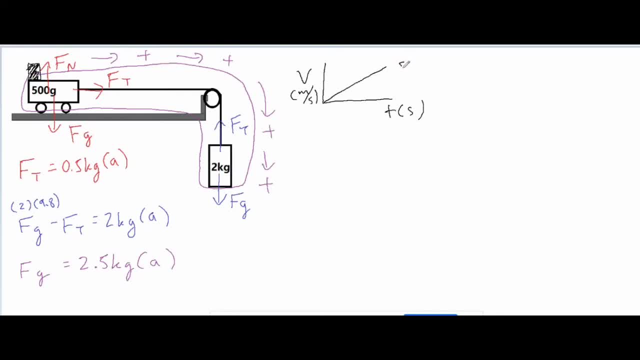 positive acceleration And let's just pretend that the slope of our line is 5 meters per second squared, Okay, then we would have our acceleration. So the first part of our video we already solved for the acceleration mathematically. So this scenario would be a little bit different, especially since there's 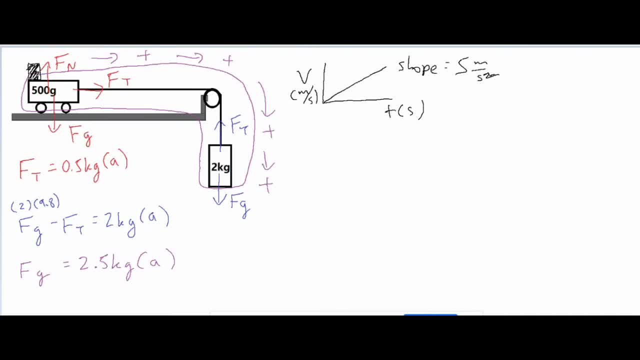 more mass on top of the cart. So we're going to take a look at the acceleration And we're going to see that our acceleration and our tension aren't going to be the same. So if we know our acceleration but there's an additional mass on top of this, we're going to have to rewrite some of our formula. 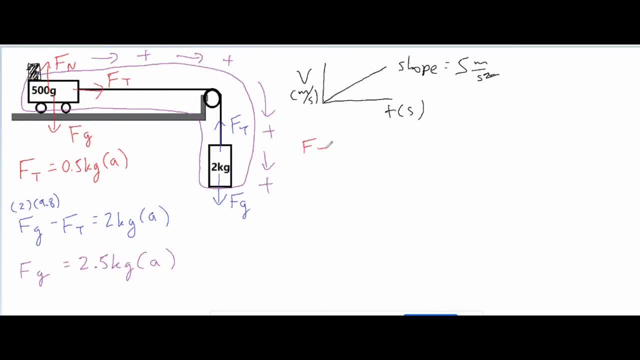 So let me go ahead and do that. We could do. Good luck, Yeah, See you guys, Bye, bye. All right, so I rewrote my red, blue and purple formula. My red one was just rewritten to include the unknown mass that is stacked on top of the 0.5 kilogram cart. My blue formula stayed the 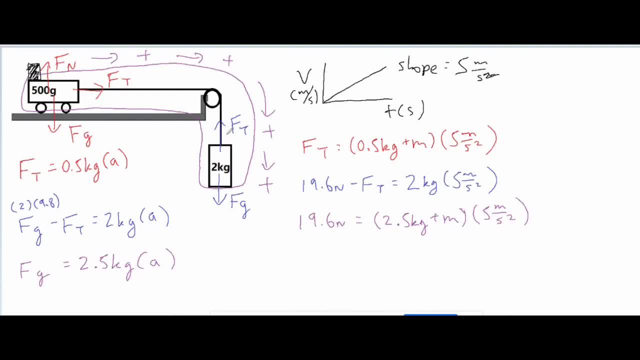 same because it doesn't involve this cart, it only involves just the hanging mass. so this still looks the same. And then for my purple formula, which is the entire system, that one is slightly different because it is that 2.5 kilograms, which is the hanging mass and the cart, and then plus. 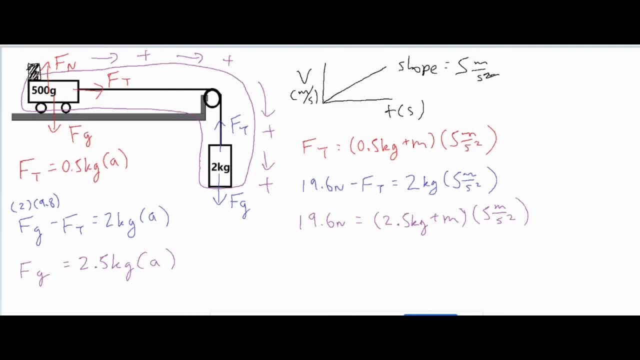 an additional unknown mass. So what we can do is we can find that unknown mass by taking a look at what we have. We have two unknowns over here. we have one unknown over here which is our FT, so we can go ahead and find FT if we wanted to, and then we have our unknown mass right over here. 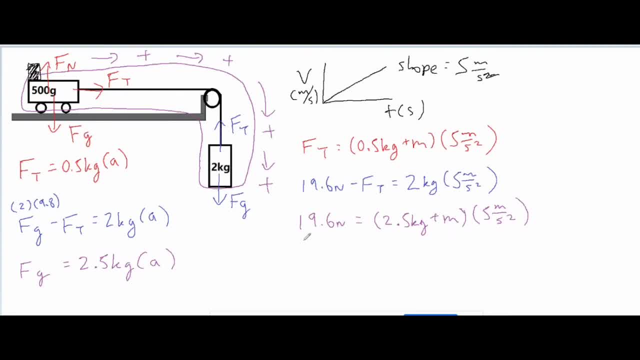 So we can go ahead and solve for our mass over here. So let's go ahead and do that, All right. so what I did is I just distributed the 5 to the 2.5.. and then the m, so i got 12.5 plus 5 times m. subtracted the 12.5 from both sides and then